12,, 14,, 16,, 18,, 20.. 2,, 4,, 6,, 8,, 10,, 12,, 14,, 16,, 18,, 20.. 2,, 4,, 6,, 8,, 10,, 12,, 14,, 16,, 18,, 20.. 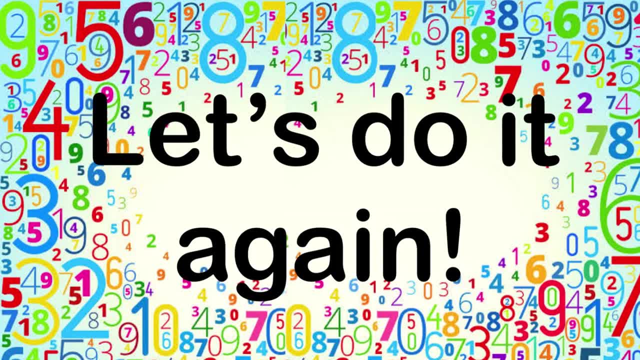 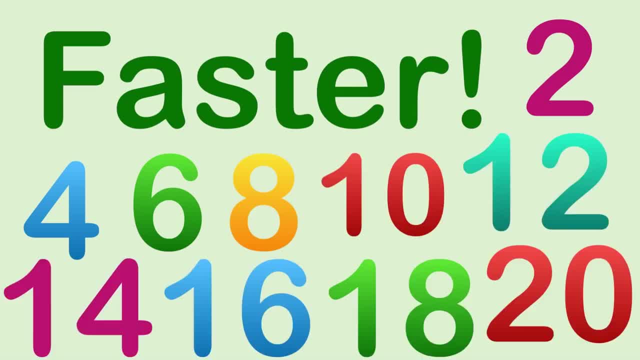 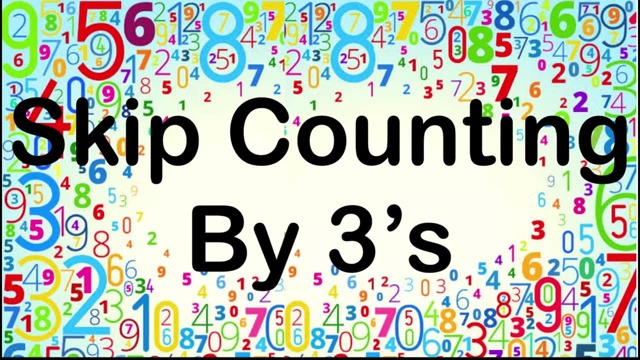 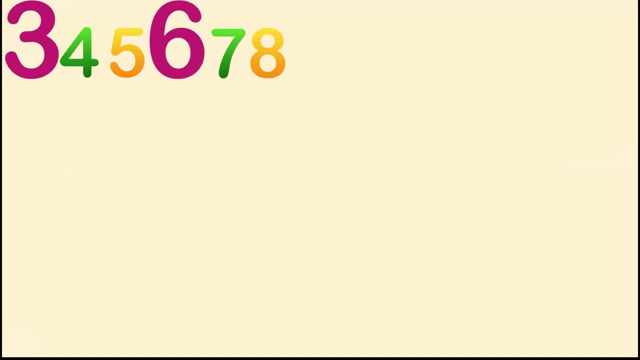 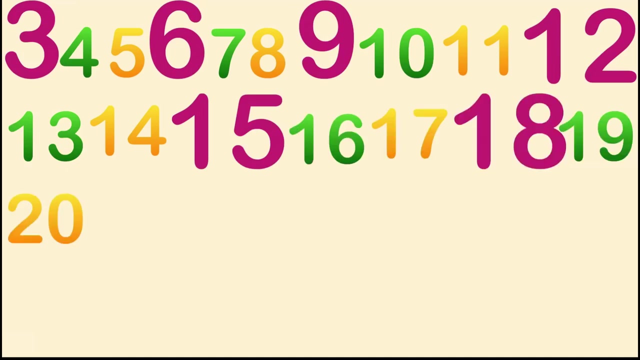 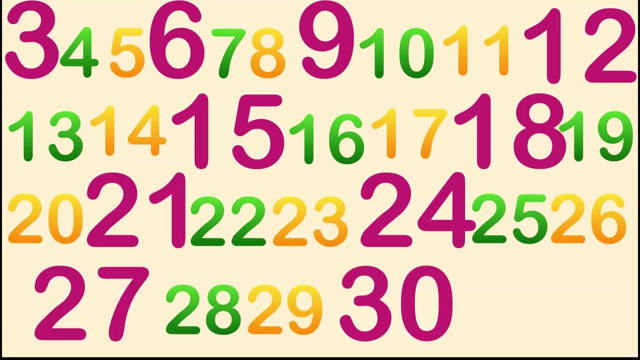 18, 20.. 2,, 4,, 6,, 8,, 10,, 12,, 14,, 16,, 18,, 20.. That is skip counting by twos. Let's go to skip counting by threes: 3,, 6,, 9,, 12,, 15,, 18,, 21,, 24,, 27,, 30.. That is skip counting by. 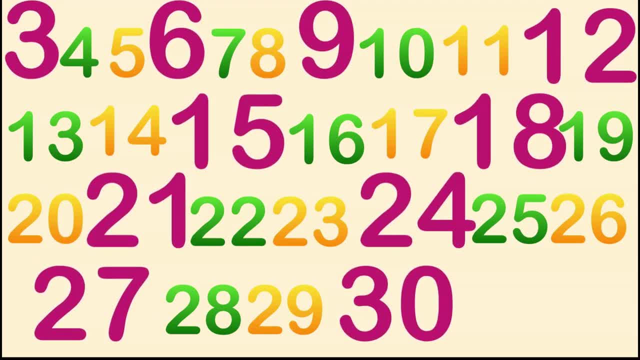 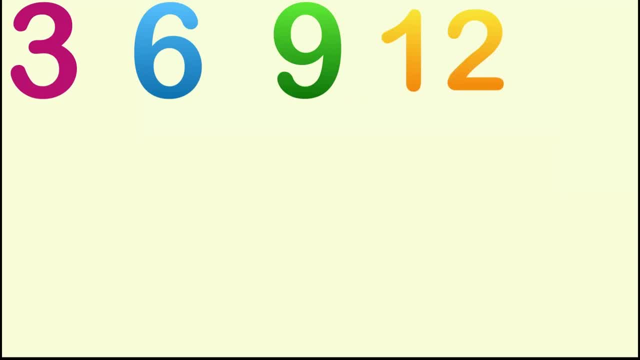 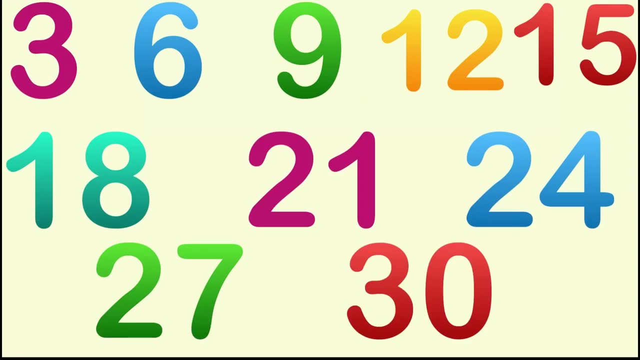 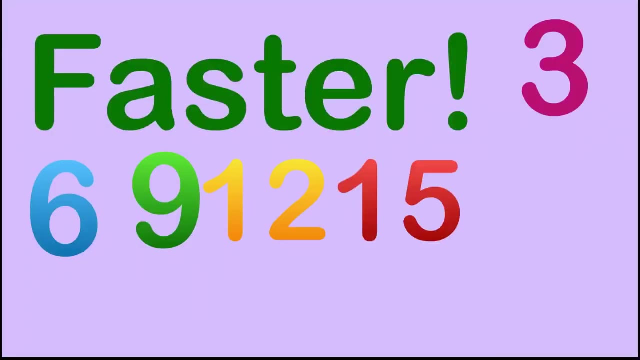 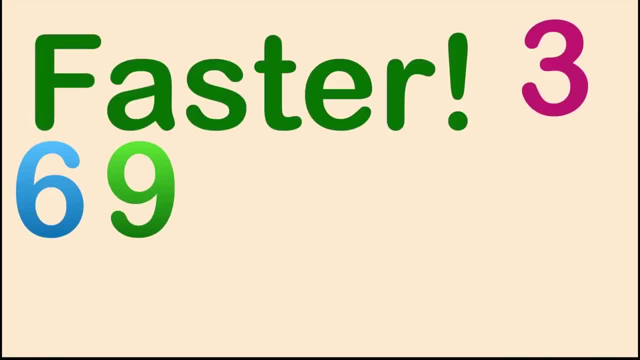 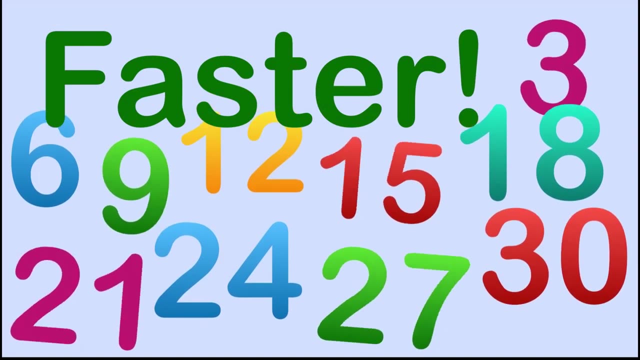 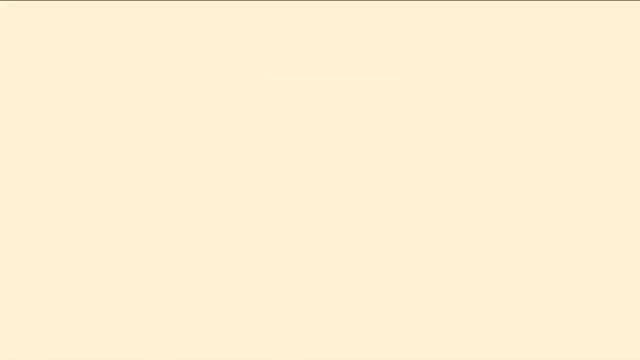 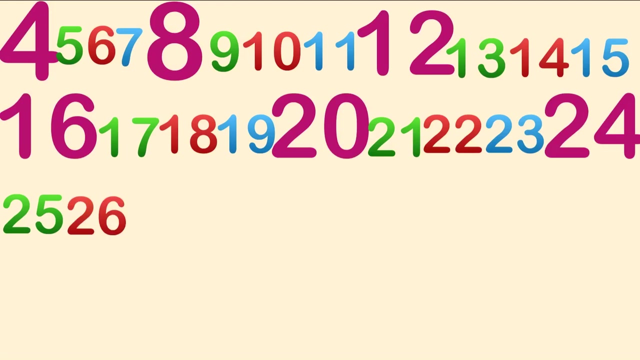 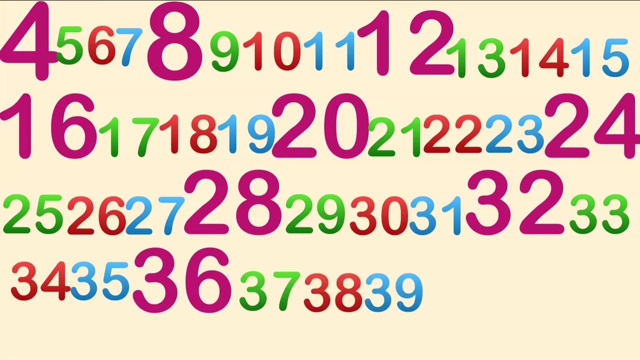 Let's go now to skip counting by fours: 4, 8,, 12,, 15,, 18,, 21,, 24,, 27,, 30.. 16,, 20,, 24,, 28,, 32,, 36,, 40. That is skip counting by fours. 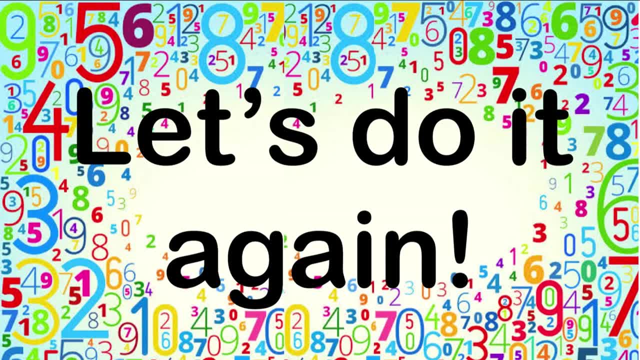 4,, 8,, 12,, 16,, 17,, 18,, 19,, 20.. Let's go now to skip counting by twos. Let's go to skip counting by threes: 3,, 6,, 9,, 12,, 15,, 18,, 21,, 24,, 27,, 18,, 21,, 24,, 27,, 30. 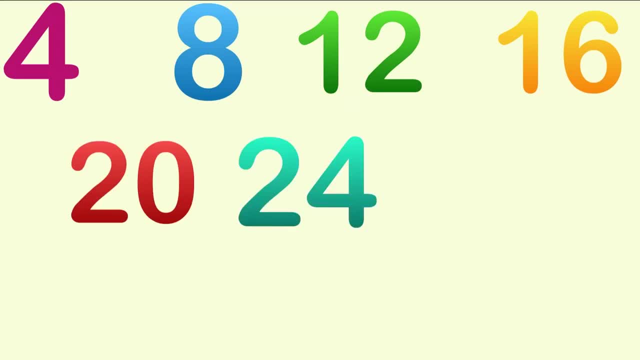 3,, 6,, 9,, 12,, 15,, 18,, 21,, 24,, 27,, 30. That is skip, counting by twos. Let's go now to 20,, 24,, 28,, 32,, 36,, 40. 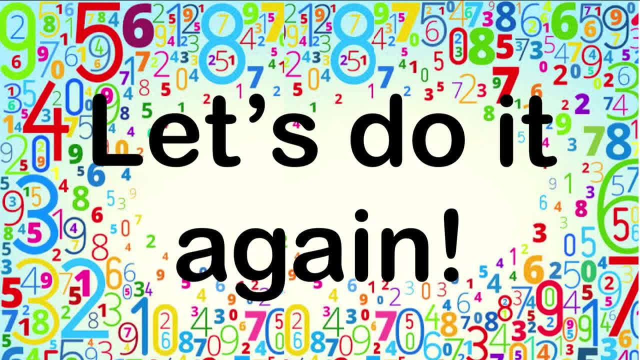 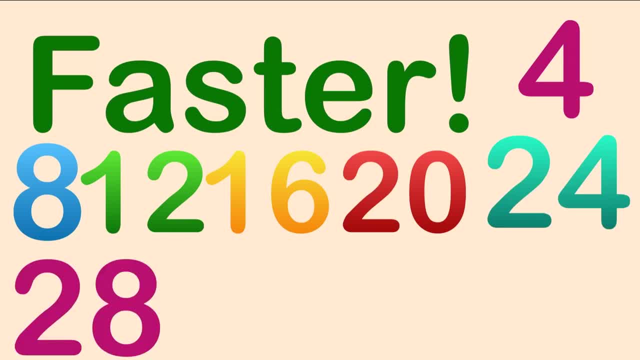 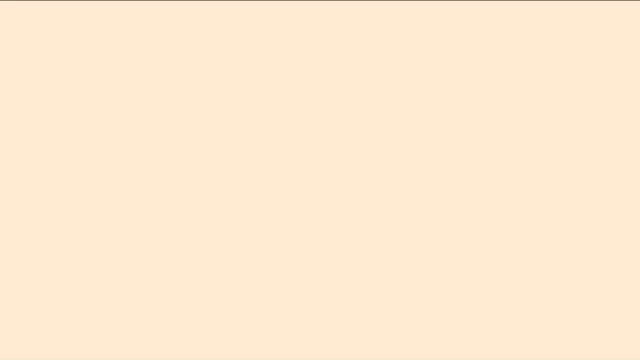 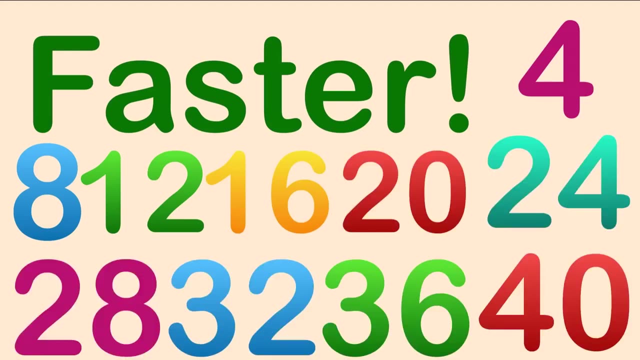 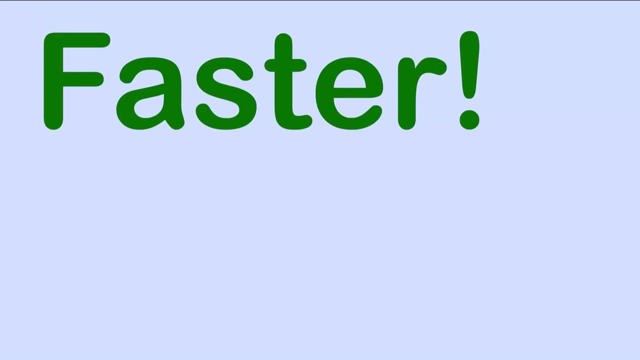 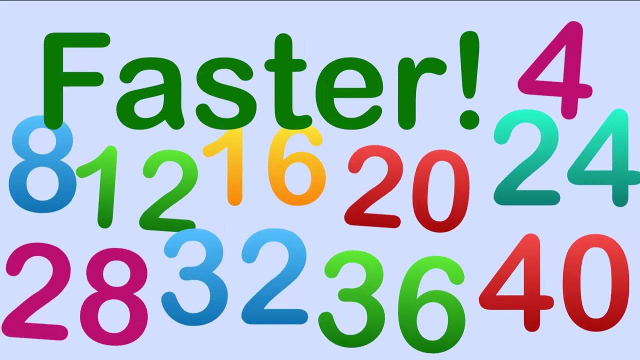 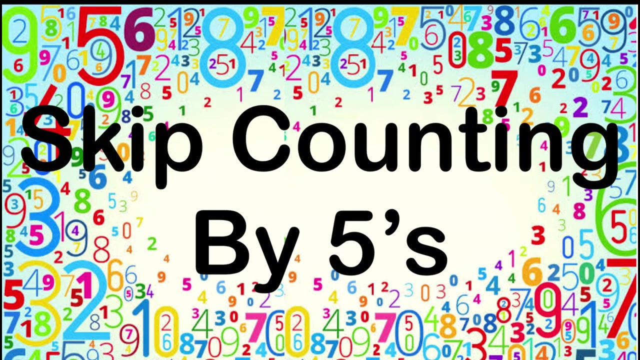 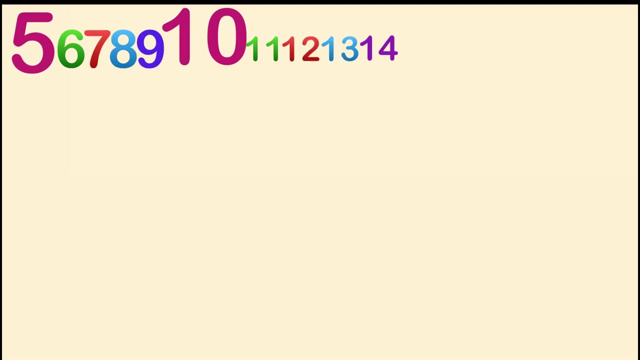 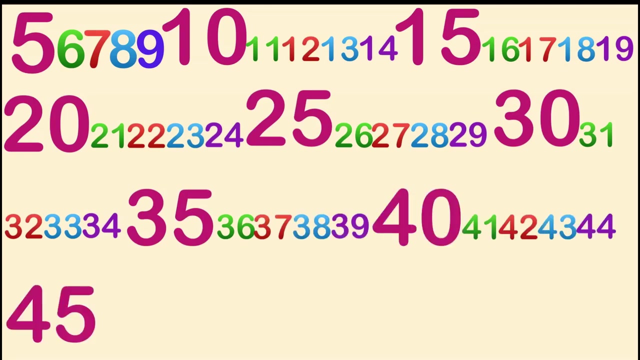 4,, 8,, 12,, 16,, 20,, 24,, 28,, 32,, 36,, 40. That is, keep counting by 4's. Let's have skip counting by 5's: 5,, 10,, 15,, 20,, 25,, 30,, 35,, 40,, 45,, 50. 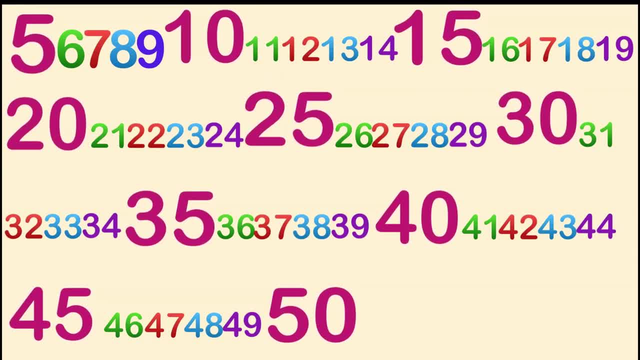 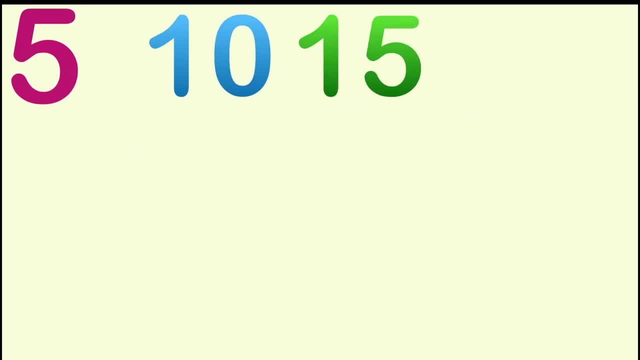 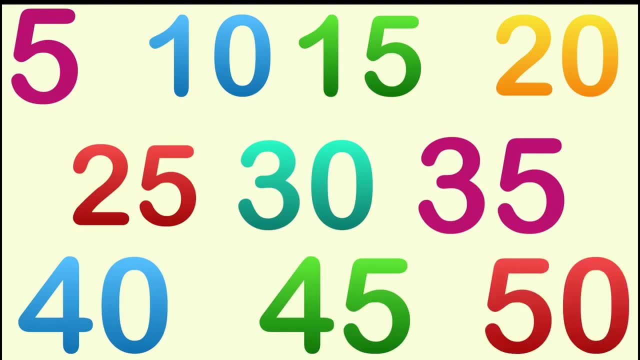 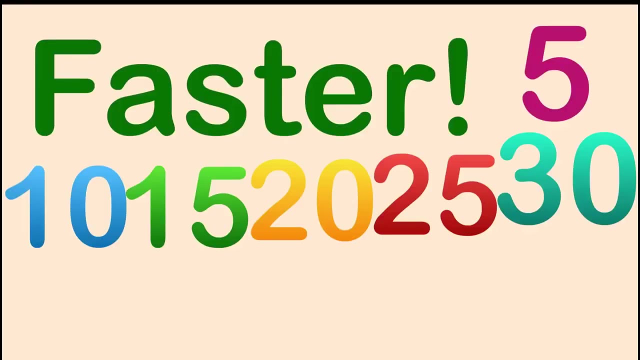 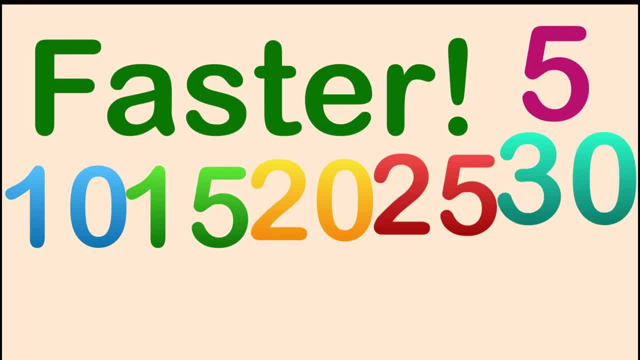 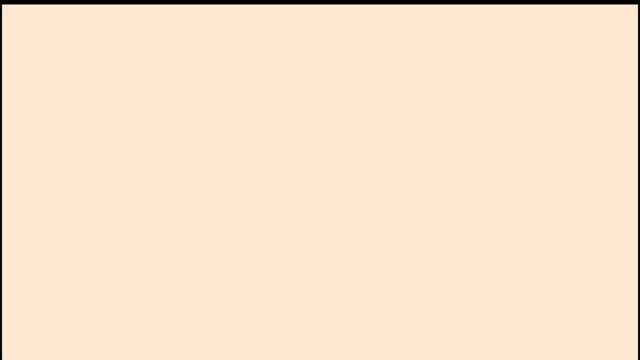 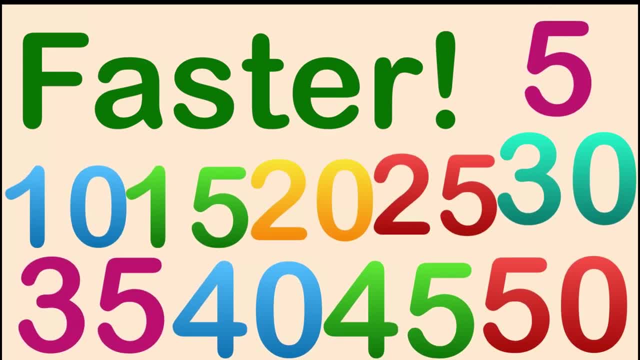 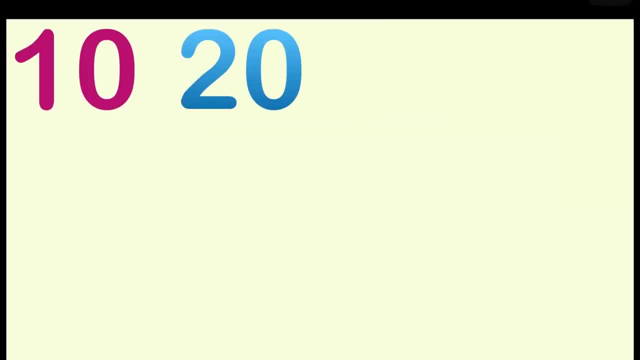 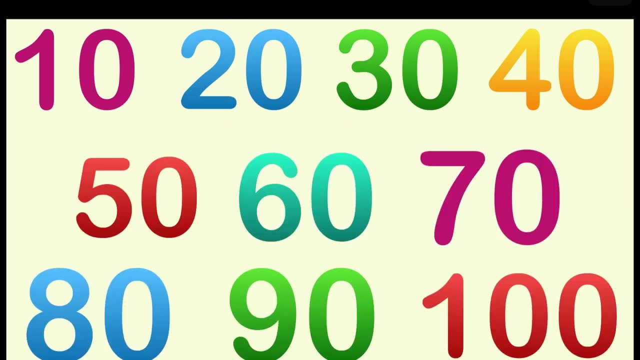 That is, keep counting by 5's. Let's go now to skip counting by 10's: 10, 20, 30, 40,, 35,, 40,, 45, 50, 60, 70,, 80,, 90, 100. 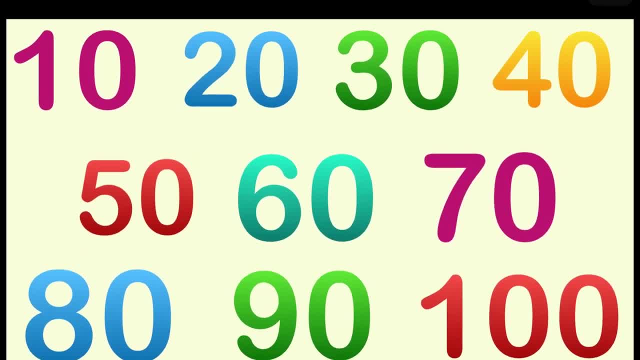 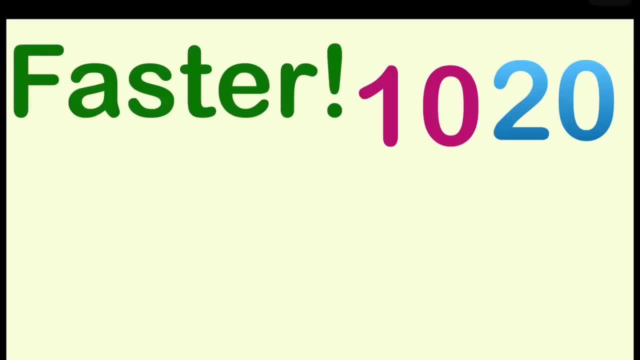 That is, keep counting by 10's: 10,, 20,, 30,, 40,, 50,, 60,, 70,, 80,, 90, 100, 10,, 20,, 30,, 40,, 50,, 60,, 70,, 80,, 90,, 100. 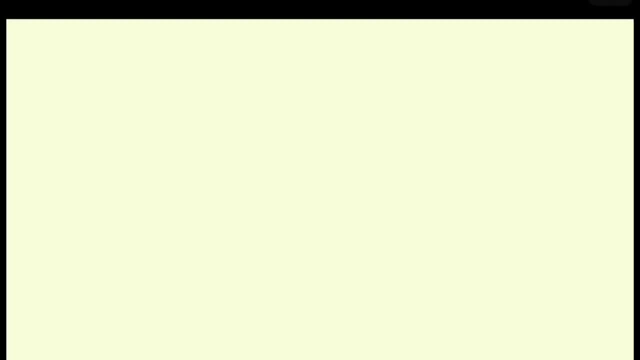 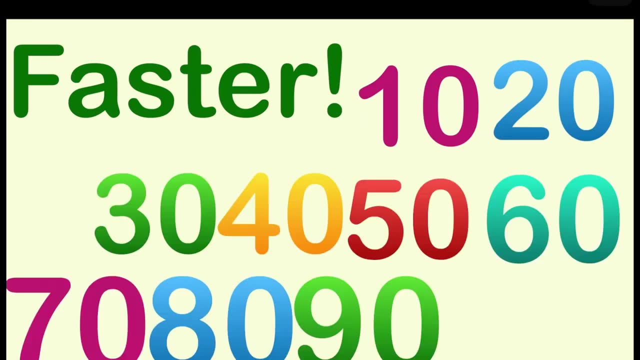 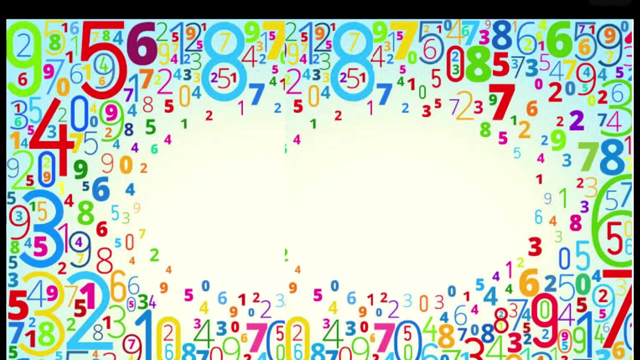 10,, 20,, 30,, 40,, 50,, 60,, 70,, 80,, 90,, 100, 70, 80,, 90,, 100.. That is, keep counting by 10s. Let's go now to skip counting by 100s. 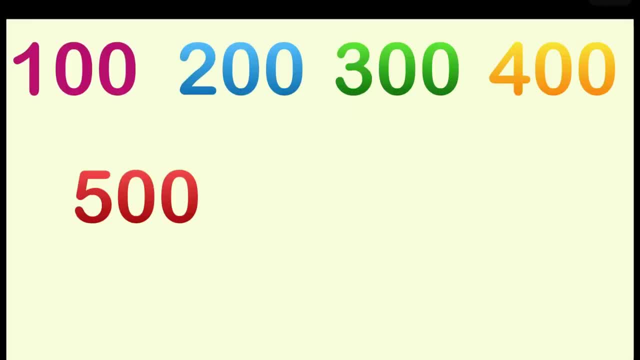 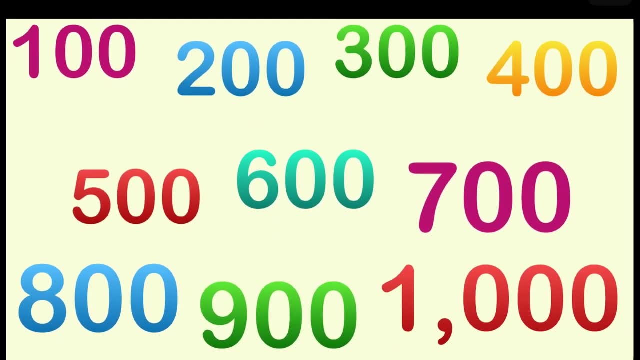 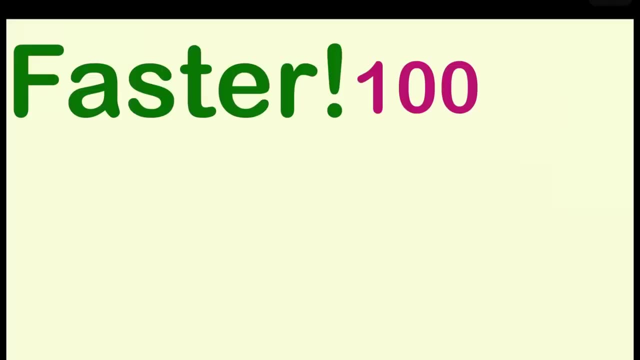 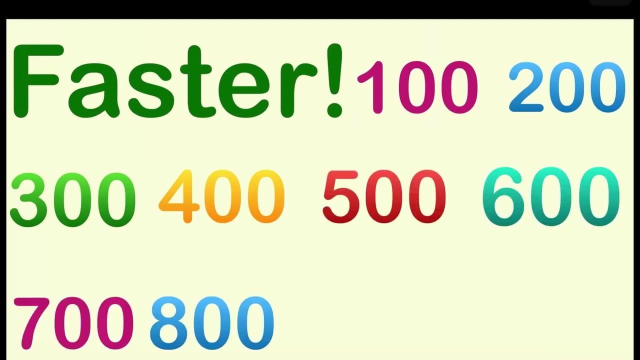 100, 200, 300,, 400, 500, 600, 700, 800, 900, 1000.. That is, keep counting by 100s: 100, 200, 300, 400, 500, 600,, 700,, 800,, 900, 1000. 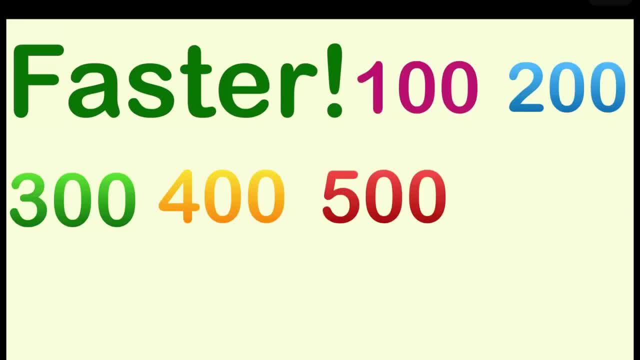 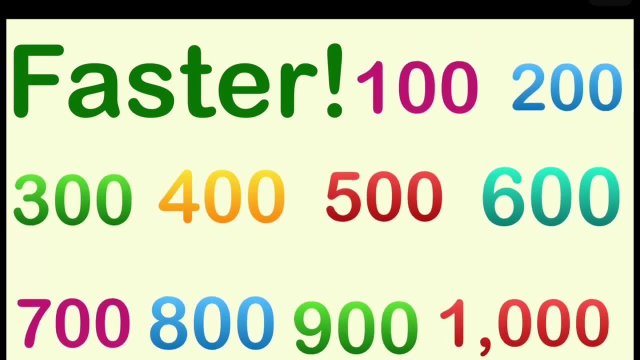 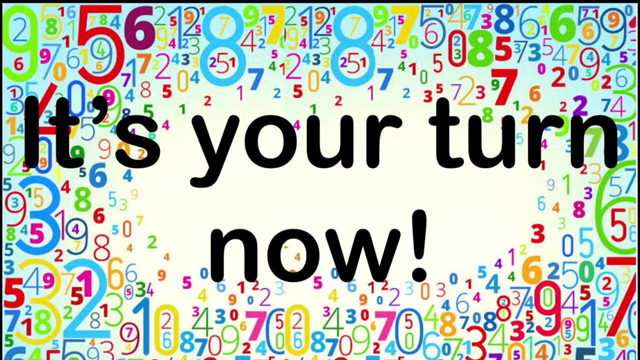 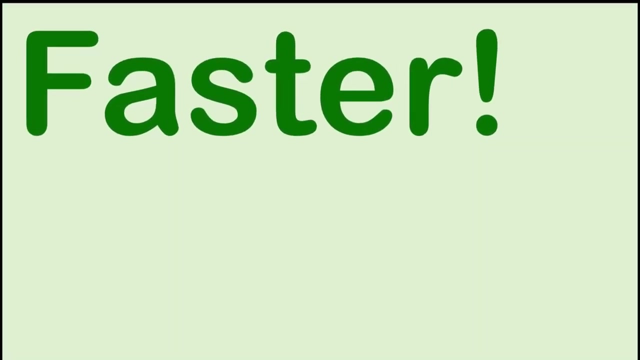 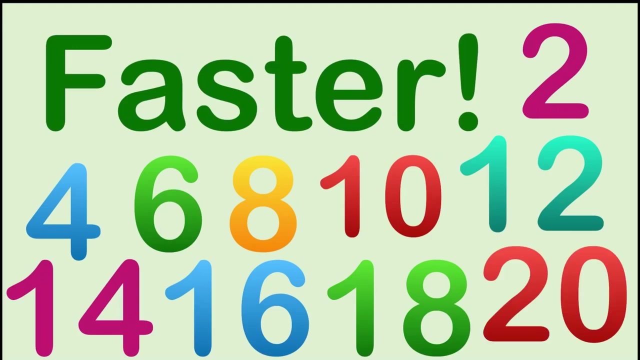 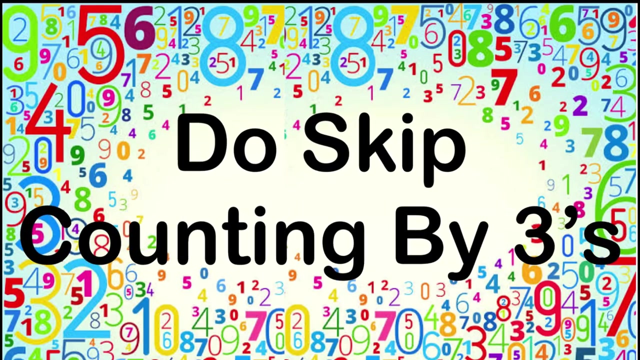 100, 200, 300, 400, 500, 600, 700, 800, 900, 1000.. That is keep counting by 100s. That is keep counting by 100s: 100, 200, 300, 400, 200, 400,, 500, 1000.